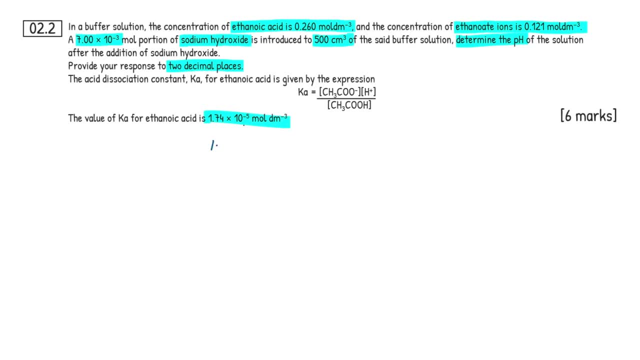 here. what is step one going to be? Any calculation question, pretty much is going to be: start with the moles. I always say this: start with moles. That's going to be our first point And we're given some variables. 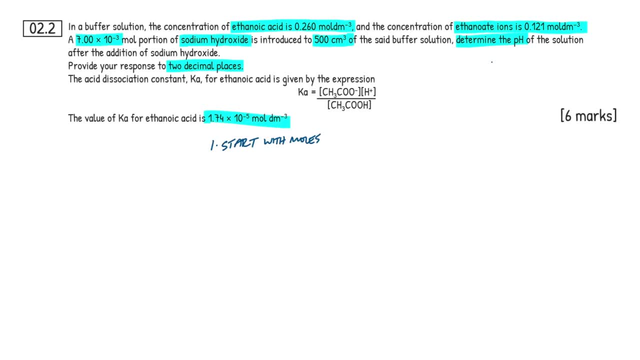 here. so it makes it really easy for us just to put it in our calculator, get it on the page and see what's going on. So what molecular equation are we going to be using here? We have n equals cv or n equals m over mr. 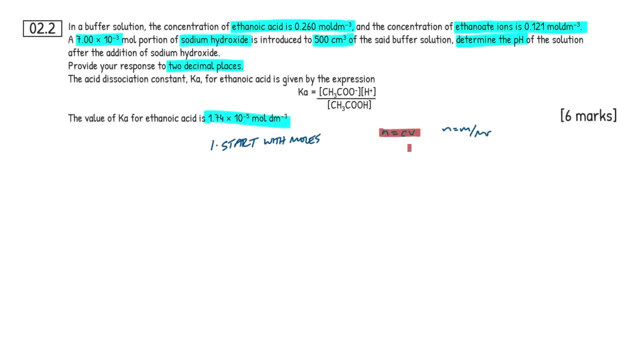 So let's look at this number here. How many moles do we want to be using Now? keep in mind: this one right here is always going to be the one that you want to use for acids and bases, just because it's always to do with a solution, right? So there's going to. 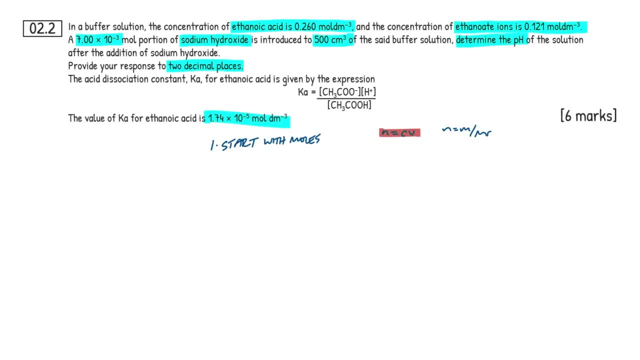 be a concentration of solution, a volume of solution, So we can use that one straight away. So what we want to think to ourselves is: what is the moles of the weak acid and what is the moles of the salt? Okay, and that's what we're going to start with, And this will 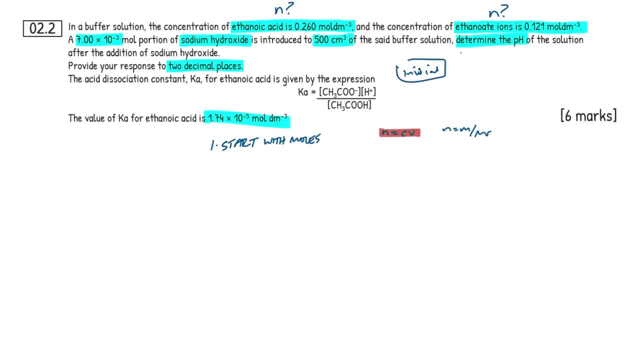 be initial okay, what's in the conical flask beaker, whatever to begin with, and then you're going to convert that into something else once you've added a acid or alkali of some kind, and that's, that's the whole point of buffers to keep the pH consistent. So let's rewrite this out: initial, final, okay, and 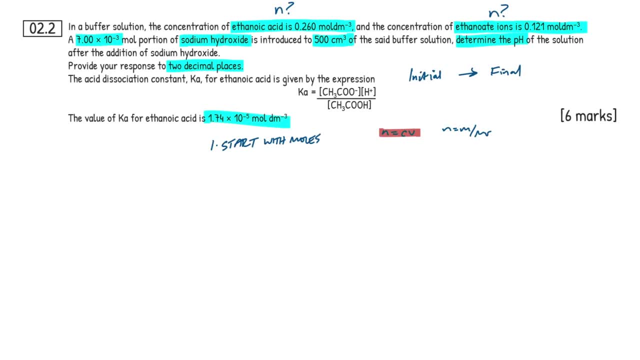 this is going to be the same with every buffer calculation and I'll sort of expand upon what I mean here. So, as I said, start with the moles. let's look at the moles of our ethanoic acid. to begin with, right COOH. This is going to be a very common weak acid that you use for these acids and bases. 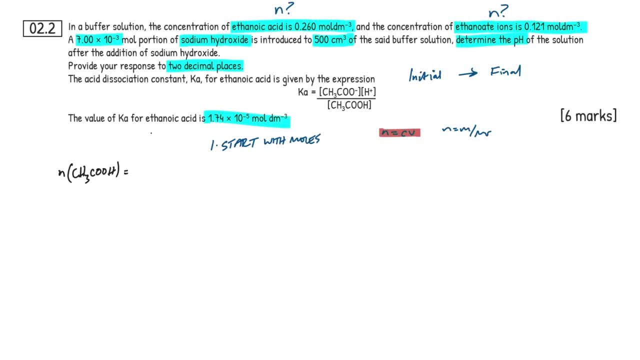 buffer calculations. So we've got a concentration here, so I'm going to use my expression. so 0.260 it's in moles per decimeter cubed, so there's no reason to convert the units. and we've got a volume of 500 centimeters cubed, okay, so all we have to do is times it by 500.. Now this is in centimeters. 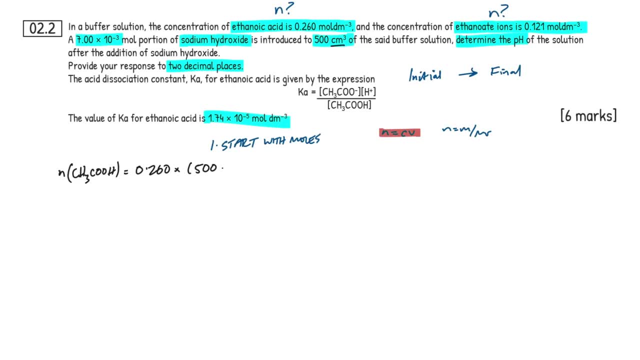 cubed, so you have to convert this into decimeters. cubed Simple times 10 to the minus 3. okay, same as divide by a thousand, up to you how you do it honestly doesn't matter. Now let's jump ahead. before we do the calculator stage, let's do the. 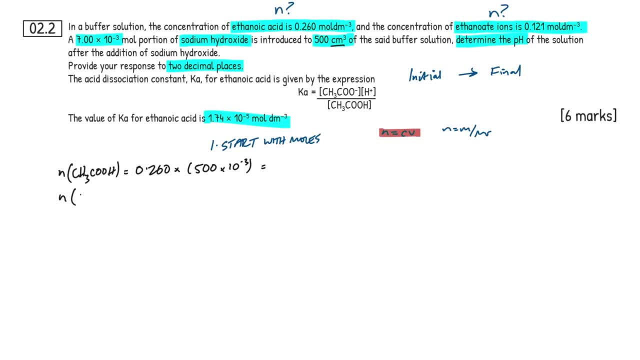 moles of the salt, the ethanoate ions next. so we're gonna have CH3COO minus. okay, so we're gonna have our concentration 0.121 multiplied by exactly the same volume. guys, it hasn't changed. okay, 500 times 10 to the minus 3.. So if you put that in your calculator and you're going to have a, 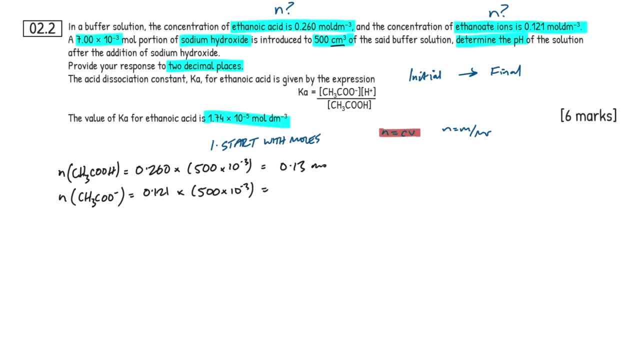 calculator, you're going to get 0.13 mole of the weak acid and 0.0605 mole of the salt. okay, that's the first two marks done. So, even if you don't really know what's going on and you're freaking out in your exam, start with the moles. okay, get yourself some marks wherever possible and just 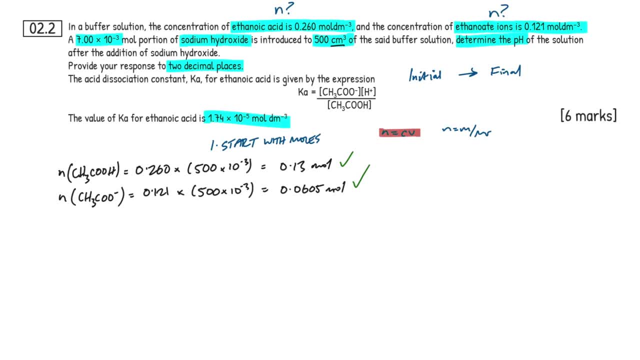 scrape through. Ideally, that's not what you want to be doing. you want to be confident with these questions, but that's just my piece of advice there. Next thing we're going to do is we're going to take the moles of the hydroxide added. we don't have to calculate it, they've given it to us. 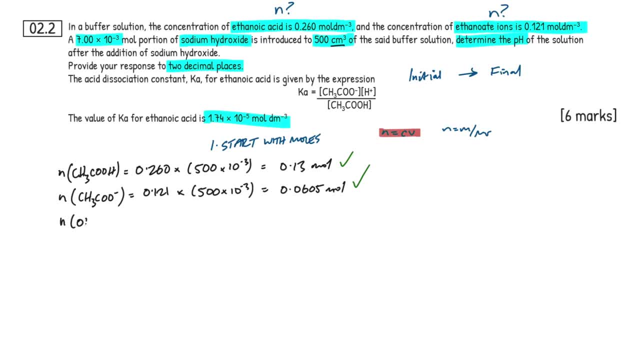 straight away in the question. okay, so I'm going to write that right here. make a note of it. moles of the hydroxide ion. that's added the strong strong base here, 7.00 times 10 to the minus 3. okay, no marks allocated here because it's given in the question. so, yeah, So we've started with the moles. 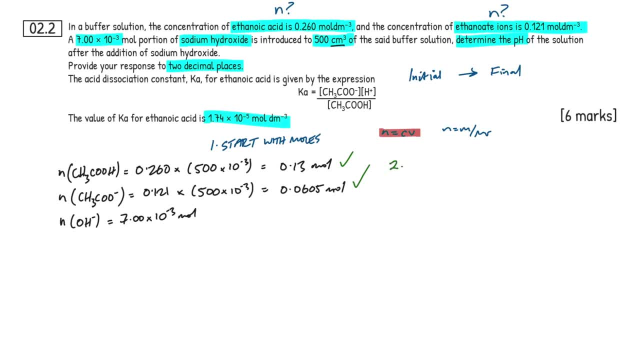 right, let's look at what step two is. so step two of any buffer calculation, this is going to be really important to remember. Okay, so, going back to what I said earlier, we're going to have moles, concentration and volume, so I'll put NCV of initial and then you're going to have moles, concentration and volume of final and 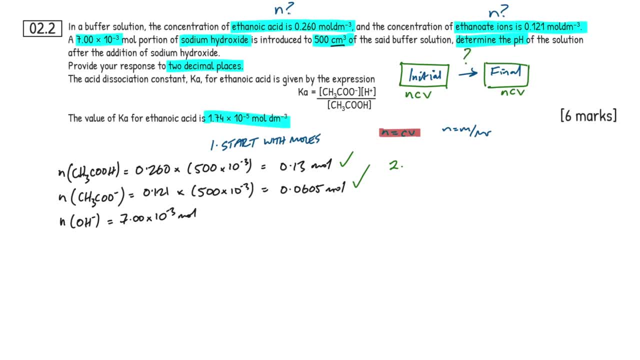 the only difference is we're adding a substance in here. okay, in this case it's a strong base, right? So, going back to step two, then let's do a little bit of theory here to so you guys can wrap your head around what's going on, and it will help you so much when it comes on. 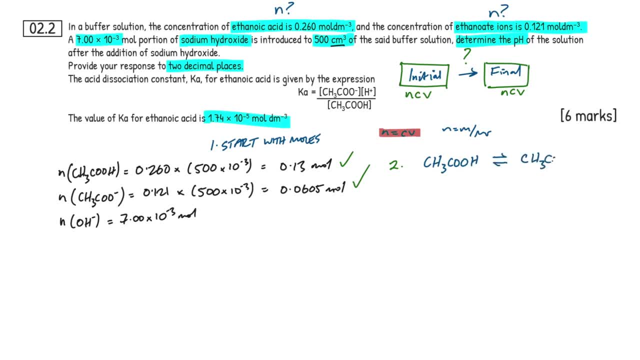 To all buffer calculations. so I'm just drawing out my equation here, plus H, plus right, so there's two options that we can have with buffers. okay, we can either add an acid to the conical flask, whatever it may be, or we can add a base or alkali, whatever you want to refer to it, as I like base, I'm just used to. 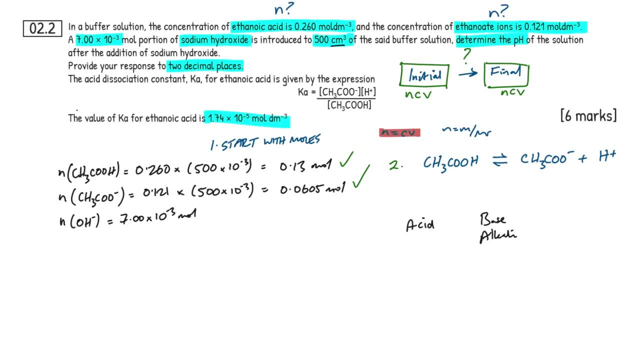 base, but you can- you can refer to it as an alkali as well. that's completely fine. now what's going to happen here is: notice this: guys Pay attention to this equilibrium symbol, okay, and that's because the equilibrium can shift. either way. it's not a strong base or a strong acid. buffers always involve weak substances, so weak acid, weak. 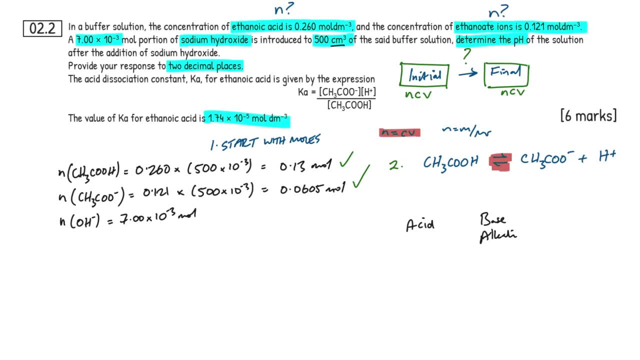 base right. so if we think about this sodium hydroxide, going back to what we added in here, we're dealing with adding an alkali in or a base, and it's a strong base. so we're going to be having our sodium hydroxide, NaOH, and we're going to have a forward. 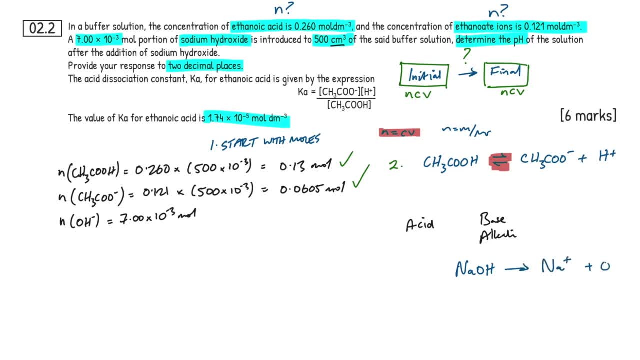 arrow. it's going to break up into its positive ion and negative anion or hydroxide. okay now, because this is a strong base, it completely dissociates we. we have an absence of an equilibrium arrow. we just have a one direction arrow and that's because the equilibrium is so far to the right. 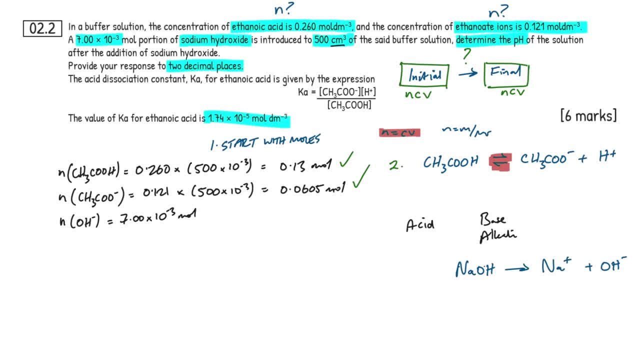 because it's completely dissociated. we can essentially think of the reactant as completely used up. okay, all we're dealing with here is our products. so what this means, then, is that adding in a strong hydroxide. we have this, this hydroxide, here, and what's going to happen is this: 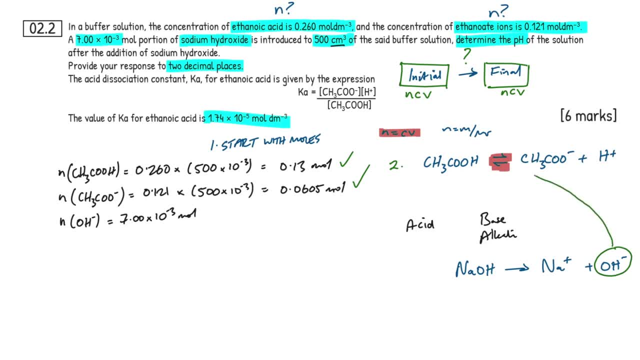 is going to be added to this solution and it's going to affect the direction of this equilibrium arrow, and that's what buffers is all about. it's all to do with equilibrium, really. so what's going to happen here? let's think about what's actually happening. so this hydroxide, this OH minus, is going. 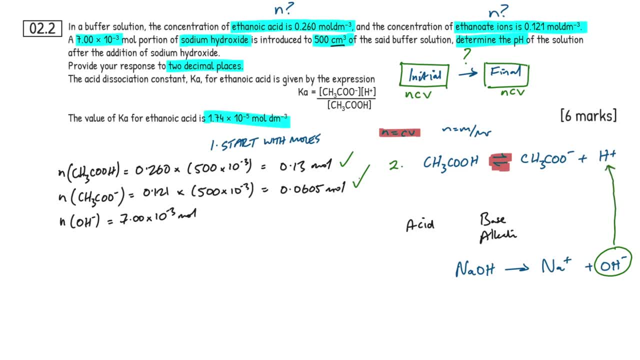 to react with this H plus. okay. so let's actually write out the second equation here. we're going to have OH minus. once it's broken down through the complete dissociation, it's going to react with the H plus and it's going to form water. okay. now, what this means is that some of this H plus has 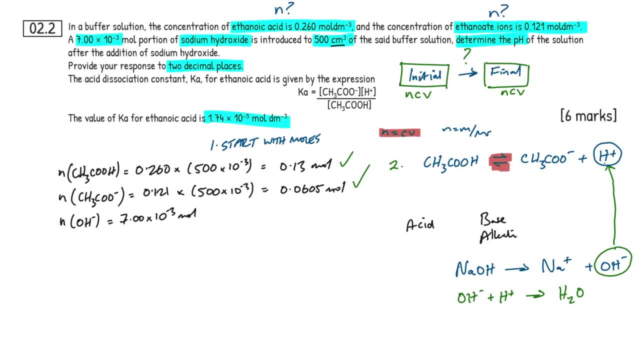 been taken away from this equilibrium to form the water. so, following Le Chatelier's principle, whatever happens to the equilibrium has to be fixed right. i know that's a super simplified version, but that's essentially how you have to think of it. you have to think of it like: 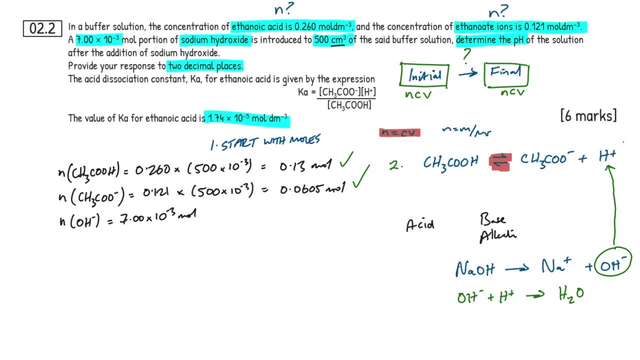 if you're adding in an H plus, you're adding in H plus. so what happens is that this equilibrium is going to shift to the right to fulfill and replace the hydrogen ions that were lost in this reaction. okay, hopefully that makes sense. now, if you're adding an acid to this right, what ultimately? 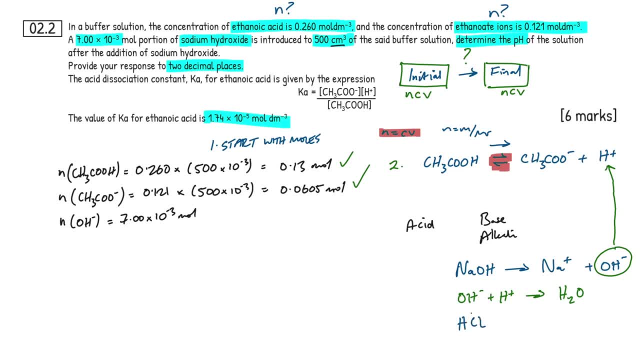 that means is like, let's say, we're adding HCl, so HCl again is a strong acid. it's going to completely dissociate into chloride ions and a proton, right. so what happens is that the proton is going to add to the the concentration or amount or moles. 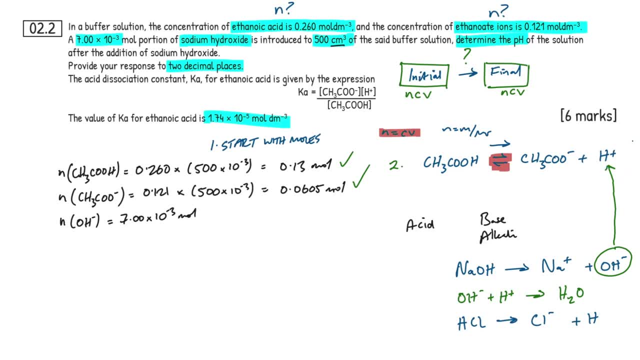 whatever you want to think of it, of the proton in this equilibrium, and to to counter that, to get it back to where it's comfortable to reach equilibrium. again, the equilibrium is going to shift to the left, okay, so just remember that buffers always relate to the equilibrium. and where is the equilibrium? 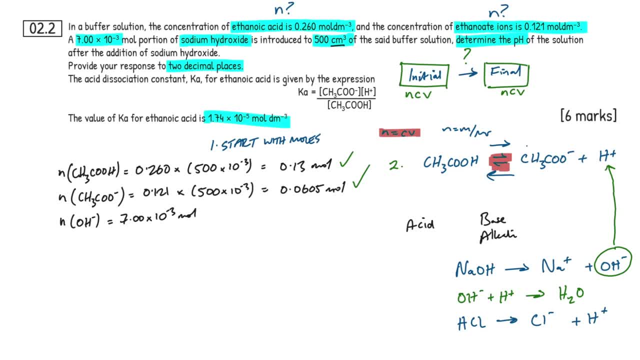 lying. okay now, if you're thinking like where the hell is he going with this? like why do i need to know this theory? so the answer is that the equilibrium is going to shift to the left for the next stage of the calculation. so i'm going to use this question as an example, but you can apply this principle to 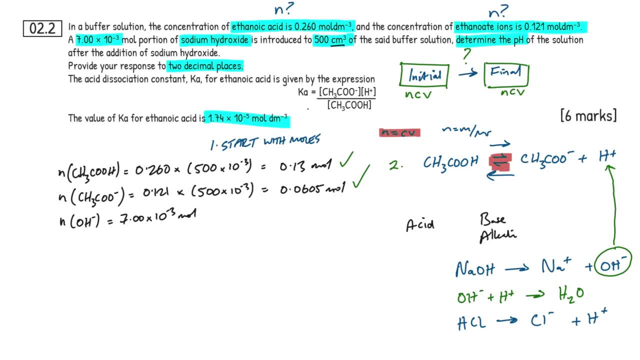 any buffer calculation question. if you want to see a question where the equilibrium shifts in the opposite direction to this question, i've already done one on my channel, so i'll link it down below. feel free to check it out. so next, then we're going to still stick with moles, okay? 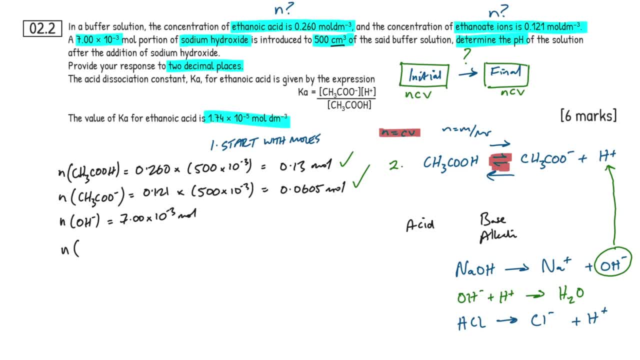 but remember i i'm sort of all over the place here, but we have initial, we have final, we've worked out. so we've, we've done this. this is initial. now we want to work out final after the strong base has been added. so let's work out what the moles of the ethanoic acid is and the moles of the salt. 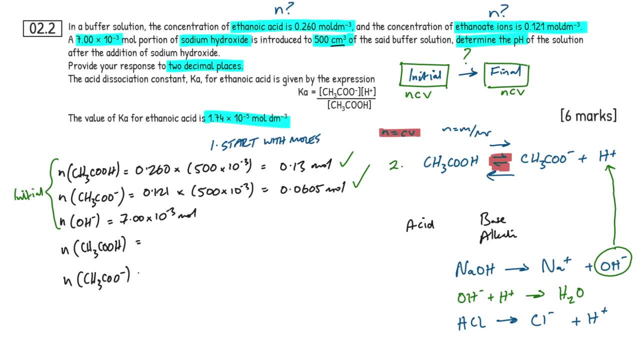 what are they going to be? so the way that this works, remember i said, when you add hydroxide is going to reactive, h plus is going to form water and the equilibrium is going to shift in this direction, in the forward direction. okay, and what that means is we have to take away the 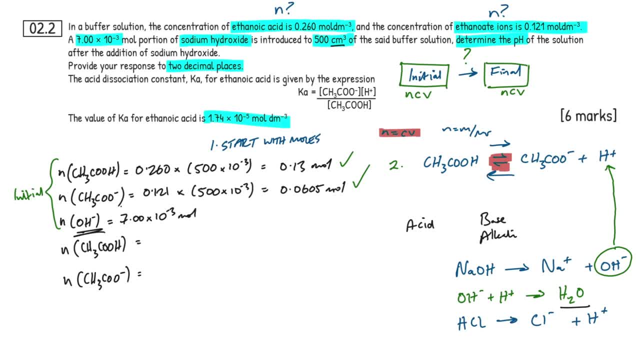 moles of hydroxide from the moles of the acid. okay, and that's because if the equilibrium is going in this direction, in the forward direction, we have to minus the moles of hydroxide that were added from the acid. if it was going in the opposite direction, you would add it onto the acid, because 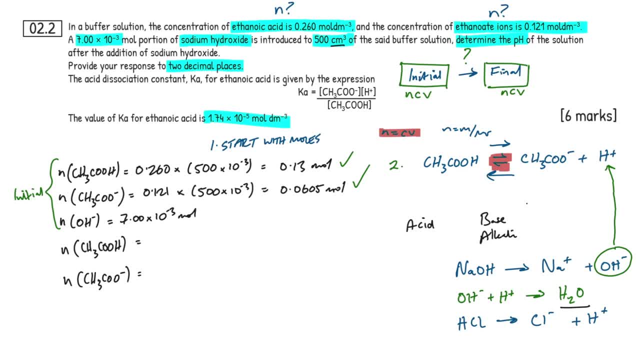 the equilibrium is going this way: um, just try and wrap your head around that practice. some questions, so much sense after a while, and it's literally just like step by step process that you apply to these calculations. so what i'm going to do here is i'm going to say, um, let's put final. 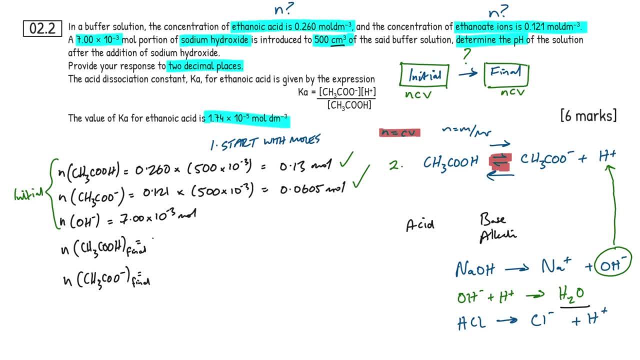 okay, remember, both of these are final after the things being at being added. so we'd have our initial moles 0.13, and we have to minus the moles of the strong hydroxide. okay, the strong base. so it's going to be 7.00 times 10 minus 3.. okay, now, equally, when we look at what is the 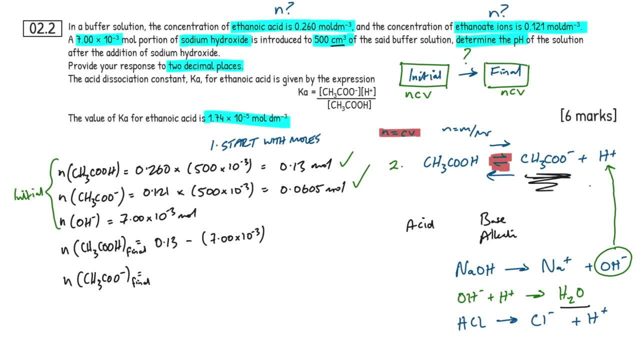 moles of the salt going to be, because it's on this side of the expression, it's in the forward direction. we have to add it on, okay, and that's again going back to the equilibrium. where is the position lying? so what we have to do is we're going to do the moles of the ethanoate originally. 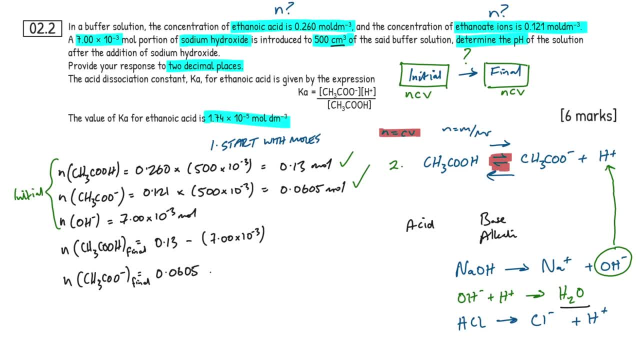 so 0.0605 plus the moles of the hydroxide, okay, so if you put both of those in your calculator, you're going to get an answer of 0.123- that's the easy one- and 0.0675- okay, so that'll be our next two moles. really try and get. 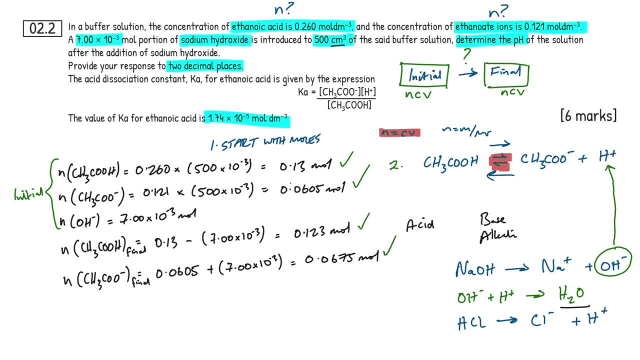 your head around the fact that if you add a base, you take, take it away from the acid, and if you add an acid, you take it away from the salt. okay, and that's because the acid is on the left of the equilibrium and the salt is on the right of the equilibrium. okay, and it's as simple as that, guys. 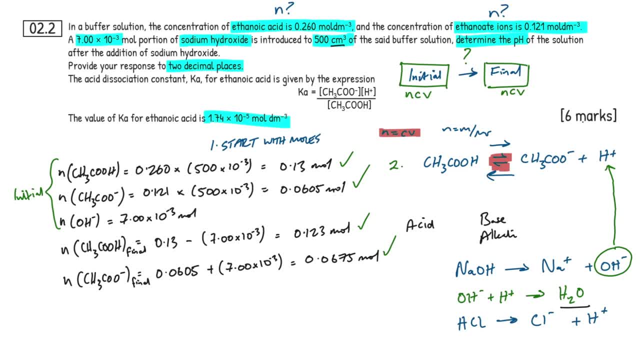 you can apply that to every single buffer calculation and make sure that you're getting those six marks okay. so next up, we have this ka expression. okay, now, every anytime you see this- they haven't just given it to you for chance and just like you know, aqa is feeling friendly. 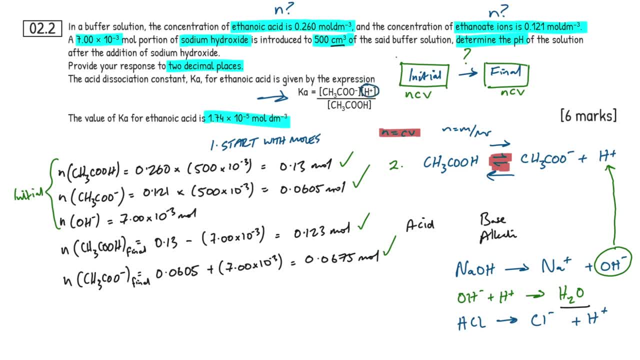 they've given it to you because you need to rearrange it to find this. okay, or maybe maybe this in a different question. you just have to rearrange it to find a specific variable and then use that to find out the ph. so if we rearrange this, then to make h plus the subject. 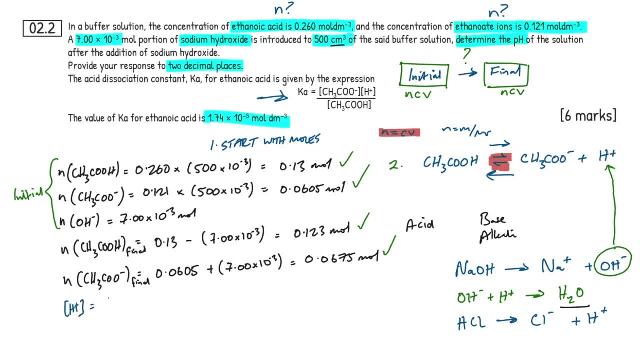 is going to become h plus equals and we're going to have ka multiplied by, and then we can just take all of this to the other side. um, so we're going to times by this, divide by this. okay, so it's going to be ethanoic acid concentration all divided by the ethanoate concentration. okay, now these square. 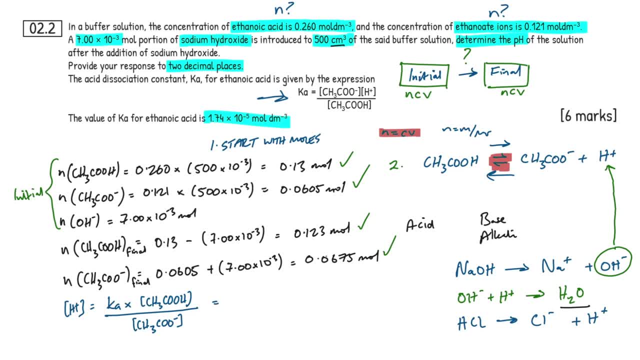 brackets, as i've said, don't know concentration. we can actually skip an entire step here and just use the moles, and the reason for that is because we have the exact same volume going on here. so if the volume like if uh, for example concentration, if we rearrange this expression, it's going to be c equals n over v, right? so if we have c equals n, 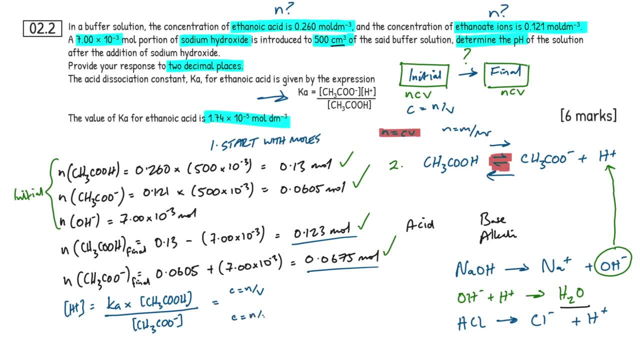 over v on the top and c equals n over v on the bottom, and the volume variables on the top and the bottom are both 500 centimeters cubed. you can cancel them out and just leave it as moles. so concentration equals moles, right, and they'll. they'll let you do that. that's completely fine. 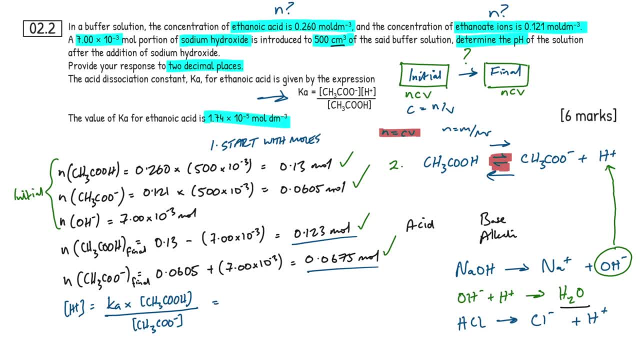 so you don't have to go to the stage of converting this into a concentration, you can just do it straight away. okay, so we have a ka value here of 1.74 times 10 to the minus 5 multiplied by our moles or our concentration. but you can do it more straight away of ethanoic acid, so 0.123. 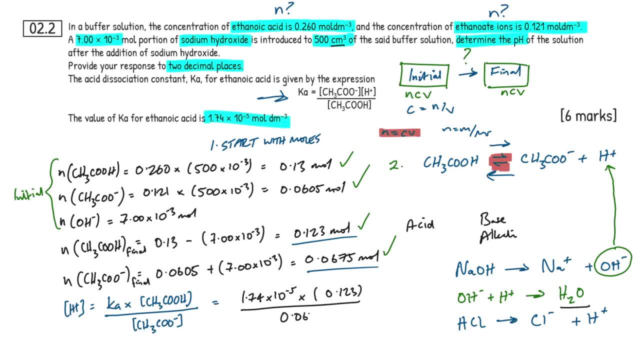 divided by this right here, so 0.0675. now, even though i could do that in this case, let's say we have a concentration of 0.047 and the volume is different on the top and the bottom- you can't do that. please always just keep that in mind in case you do have to formally work out what the 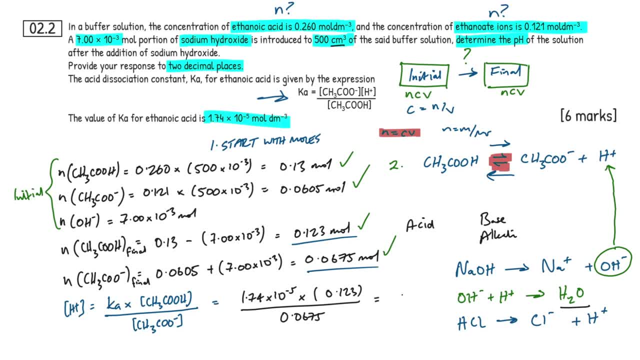 concentration is: don't skip a step when you can't and then just lose silly marks. so this is going to be 3.17 times 10 to the minus 5 once you put that in your calculator. okay, so we have a h plus concentration. all we have to do here is plug it into our ph expression. do you remember what the ph? 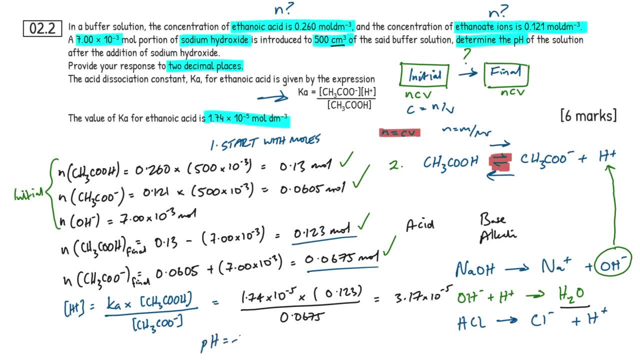 expression is. it's a real simple one. so that's going to be 0.148 plus 5 equals minus log h plus concentration. okay, so all we have to do then i'm actually going to rub this h plus concentration out and put in our actual value. 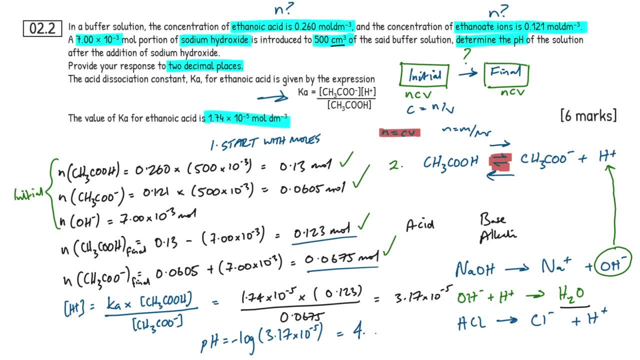 um, it's going to be 3.17 times 10 to the minus 5.. put that in your calculator. you're going to get an answer: a long ass number: 4.49894, dot, dot, dot. right, what, how many decimal places do we want we? 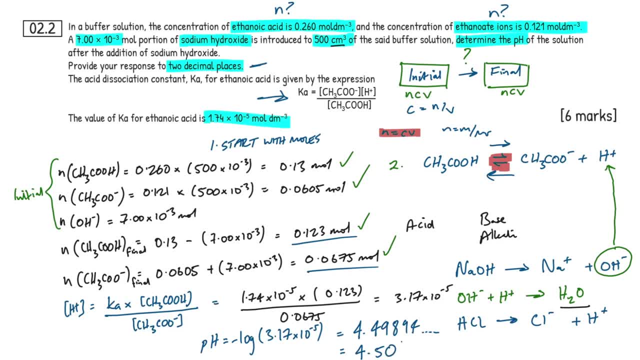 It's going to be 4.50, okay, So the fifth mark would come from working out the H plus concentration, and the sixth and final mark would be from the pH to two decimal places. So six marks in the bag, not too bad. 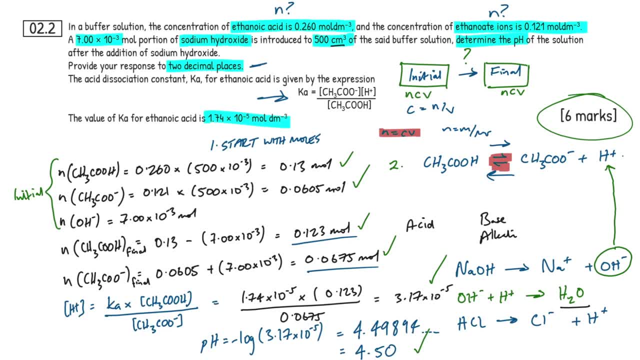 So let's quickly, before I wrap up the video, go for the examiner's report. This is an incredibly useful resource that not too many students use, so try and use it more often if you can. if you're really going for those A's A stars. 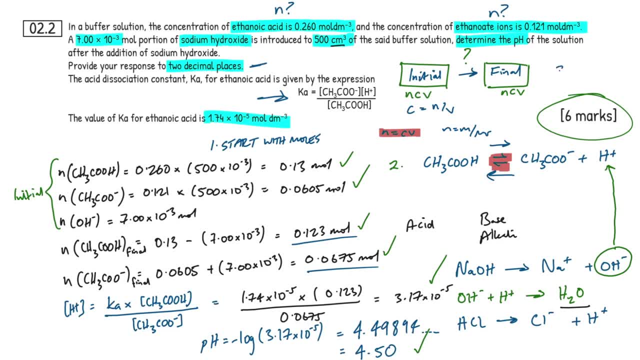 So how many students got six marks here? Thirty-four percent. okay, Thirty-four percent got six marks, which is surprisingly good, but hopefully, if you watch my videos, 100% of you that do this should get four marks. Fingers crossed. 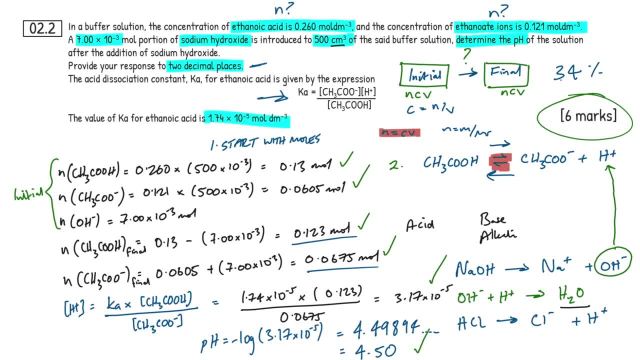 So what else did the examiner's report say? It says common errors involved failure to add or subtract the correct amount in moles of sodium hydroxide, or to subtract or add in the wrong way. So they may have added the moles of the strong base here. 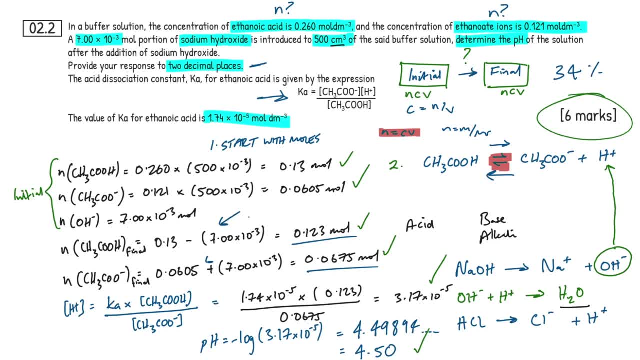 and subtracted, Or subtracted it from the salt instead. Really try and understand the theory that I detailed in step two and you should be completely fine, okay, So just pay attention In the question: is an acid added or is an alkali added or a base, however you want to refer to it as?